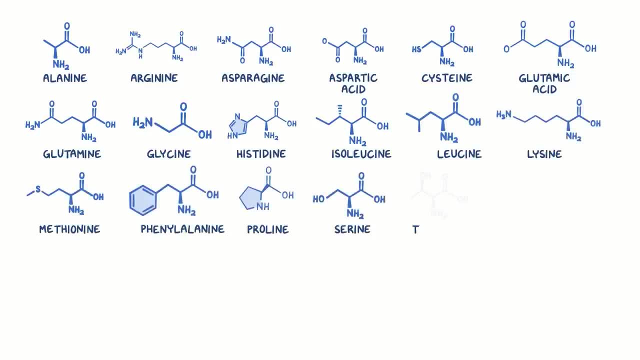 glycine, methionine, phenylalanine, proline, serine, threonine, tryptophan, tyrosine and valine. That's 20.. One way to divide them is by defining which ones our bodies can make and which ones we. 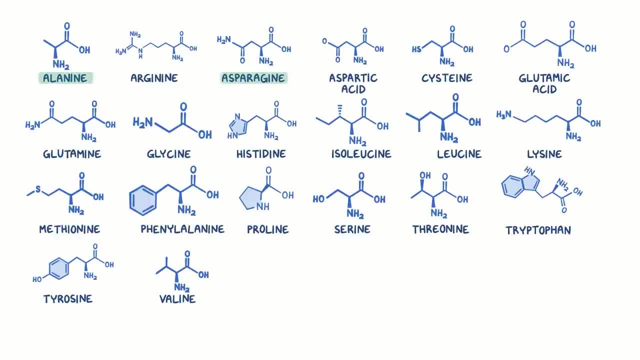 can't. There are five amino acids- alanine, asparagine, aspartic acid, glutamic acid and serine- that we can get from foods, but we can also make ourselves. These are called non-essential amino acids. 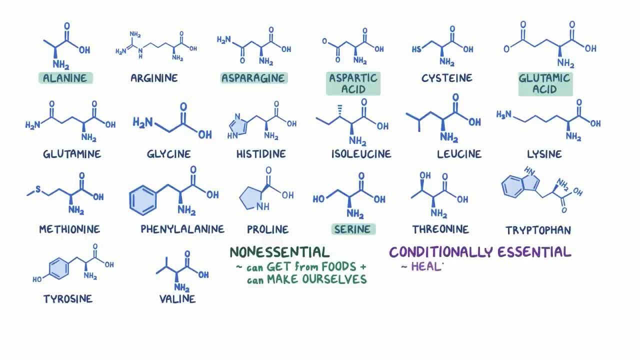 Then there are six that we call condensates. These are called non-essential amino acids. Then there are six that we call condensates. Then there are six that we call condensates. For example, a few mild amino acids: arginine, cysteine, glutamic acid, glycine, proline. 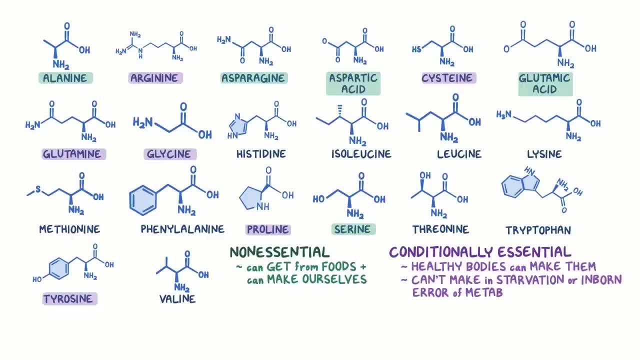 tyrosine. However, we can't make them in cases like starvation or certain inborn errors of metabolism. Finally, there are nine of them that we can only get from food: Histidine, isoleucine, leucine, lysine, methionine, phenylalanine, threonine, tryptophan and valine. We call 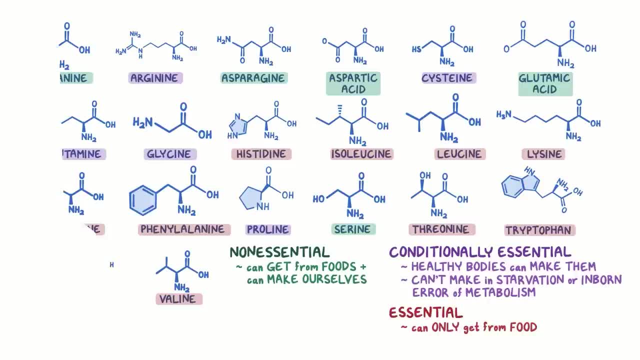 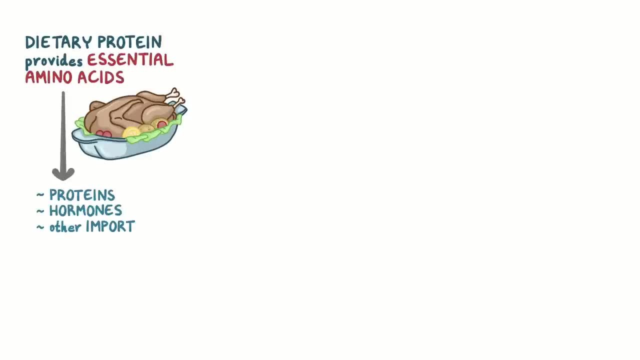 these the essential amino acids. essential amino acids: Dietary protein provides the essential amino acids that are needed to make our own proteins, hormones and other important molecules a circle of life of sorts. But to do so we need to break the dietary protein down first through a process called. 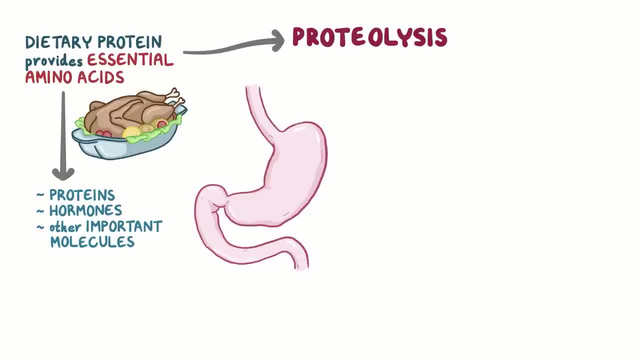 proteolysis When we first eat a protein-containing food. proteolysis begins when the food reaches the stomach First. hydrochloric acid denatures the protein, unfolding it and making the amino acid chain more accessible to enzymatic action. 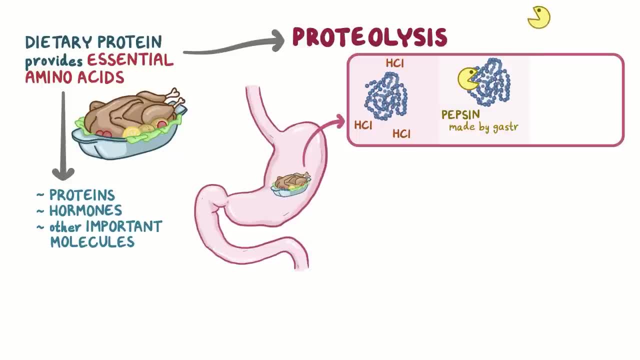 Then pepsin, which is a protein itself made by gastric chief cells, enters the picture. Pepsin cleaves any available protein into smaller oligopeptide chains which move into the duodenum, where a second set of digestive enzymes made by the pancreas further chop. 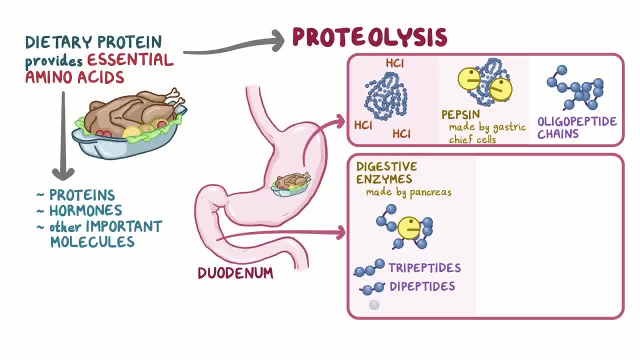 the oligopeptides into tripeptides, dipeptides and individual amino acids. These can all be taken up to the intestinal cells, where di- and tripeptides are then converted into amino acids. Some amino acids remain in these cells and are used to synthesize intestinal enzymes. 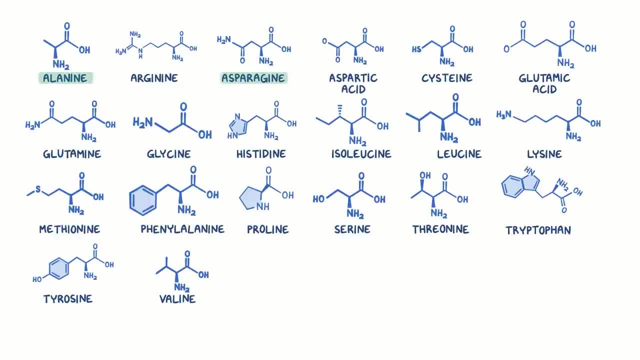 can't. There are five amino acids- alanine, asparagine, aspartic acid, glutamic acid and serine- that we can get from foods, but we can also make ourselves. These are called non-essential amino acids. 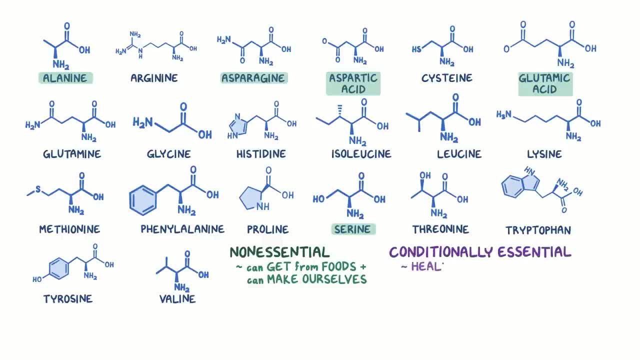 Then there are six that we call condensates. These are called non-essential amino acids. Then there are six that we call condensates. Also, condensates are known to be extertially essential because healthy bodies can make them under normal circumstances: arginine, cysteine, glutamine, glycine, proline and 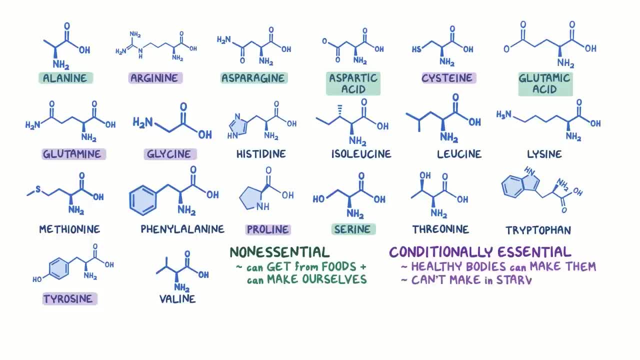 tyrosine, but we can't make them in cases like starvation or certain inborn errors of metabolism. Finally, there are nine that we can only get from food: histidine, isoleucine, leucine, lysine, methionine, phenylalanine, threonine, tryptophan and valine. We call these the. 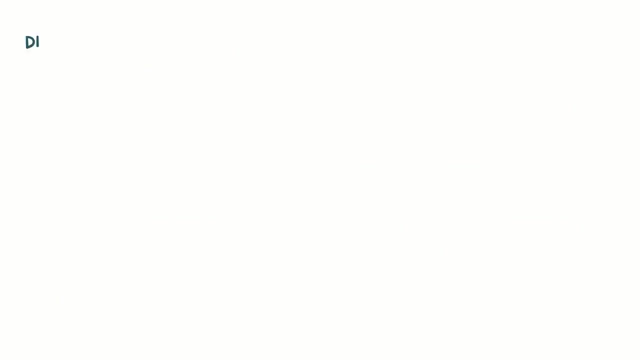 essential amino acids. Dietary protein provides the essential amino acids that are needed to make our own proteins, hormones and other important molecules a circle of life of sorts. But to do so we need to break the dietary protein down first, through a process called 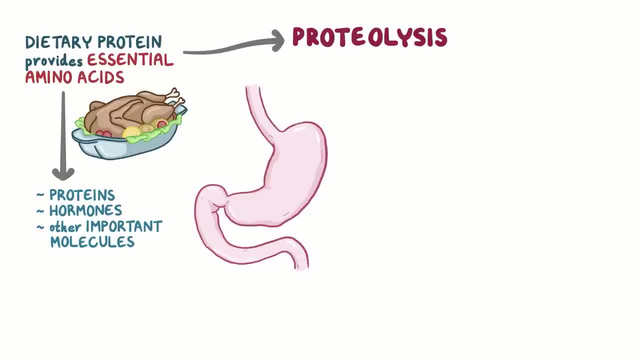 proteolysis When we first eat a protein-containing food. proteolysis begins when the food reaches the stomach First. hydrochloric acid denatures the protein, unfolding it and making the amino acid chain more accessible to enzymatic action. 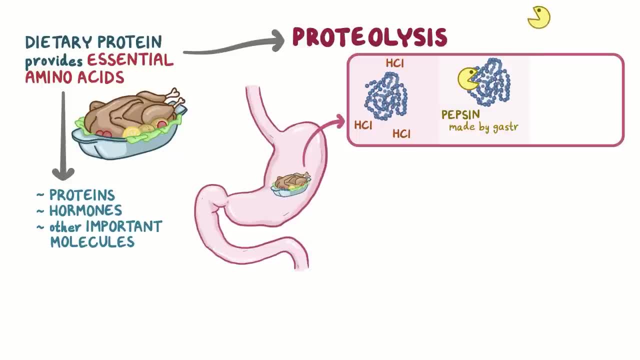 Then pepsin, which is a protein itself made by gastric chief cells, enters the picture. Pepsin cleaves any available protein into smaller oligopeptide chains which move into the duodenum, where a second set of digestive enzymes made by the pancreas further chop. 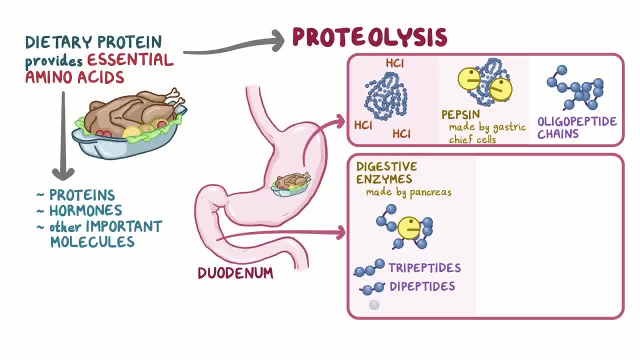 the oligopeptides into tripeptides, dipeptides and individual amino acids. These can all be taken up to the intestinal cells, where di- and tripeptides are then converted into amino acids. Some amino acids remain in these cells and are used to synthesize intestinal enzymes. 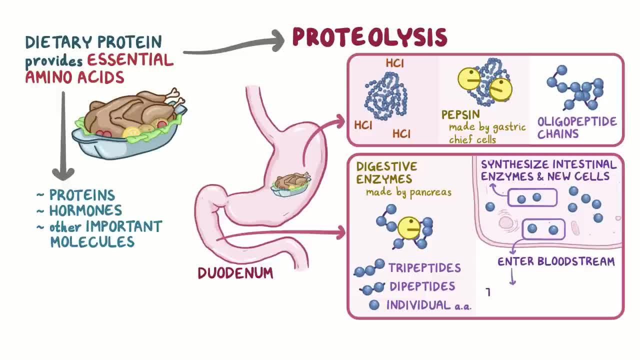 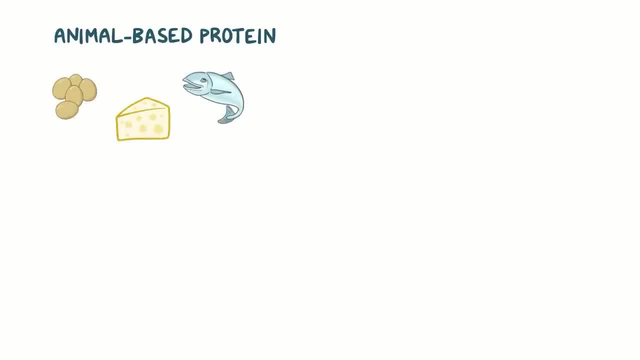 and new cells, But most enter the bloodstream and are transported to other parts of the body. In general, animal-based protein foods like eggs, dairy seafood and meat provide all nine essential amino acids in adequate amounts. Soy foods are unique in that they are plant-based and also provide all nine essential amino. 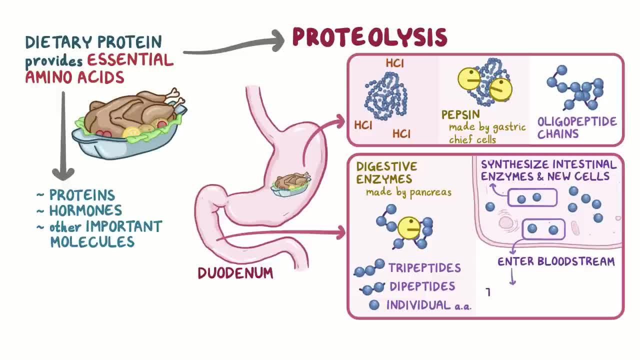 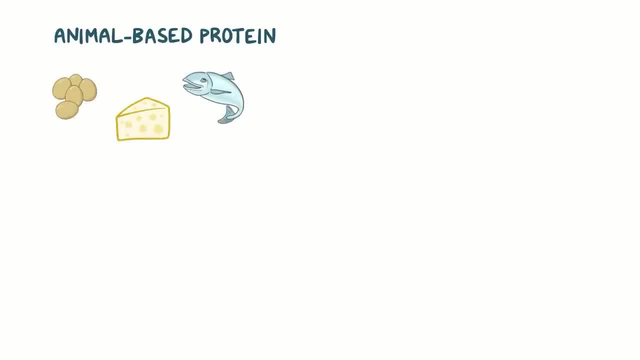 and new cells, But most enter the bloodstream and are transported to other parts of the body. In general, animal-based protein foods like eggs, dairy seafood and meat provide all nine essential amino acids in adequate amounts. Soy foods are unique in that they are plant-based and also provide all nine essential amino. 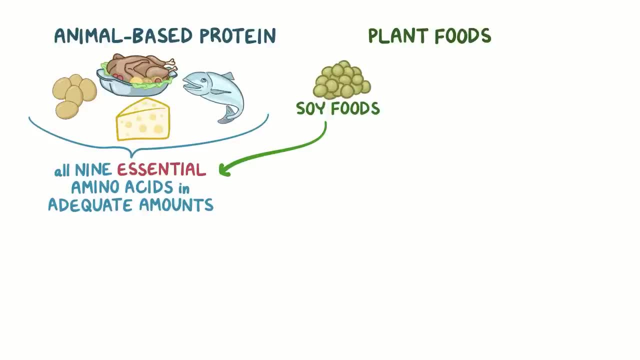 acids in adequate amounts. Most other plant foods, including whole grains, legumes, nuts and seeds, have high amounts of some amino acids and low amounts of others. Hearing this, it might be easy to assume that animal-based foods provide more protein than 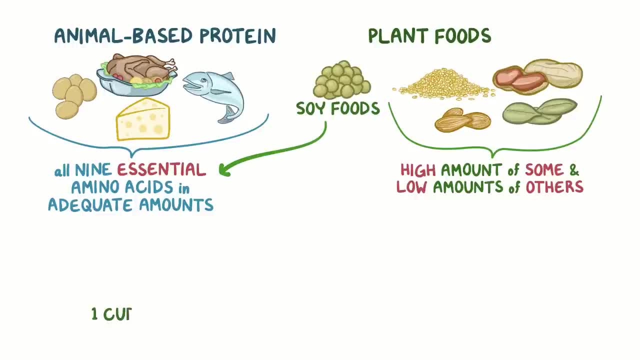 plant-based ones. But, as it turns out, a cup of tofu has the same number of grams of protein as three ounces of steak, chicken or fish, And half a cup of lentils has more grams of protein than an egg. And not all plant foods are low in the same amino acids, so eating a variety of plant-based 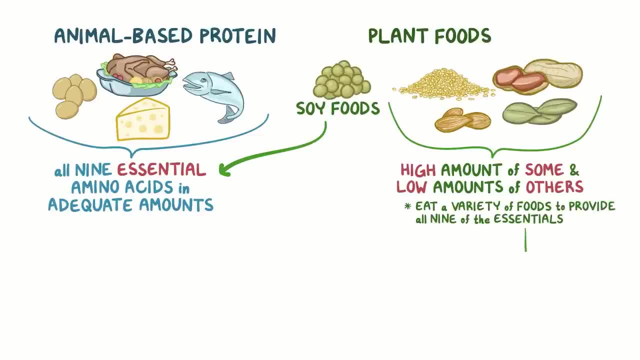 foods can provide all nine of the essentials, For example, pairing protein sources like rice and beans or hummus and pita bread or oatmeal topped with almond butter. However, in terms of volume, it may be necessary to eat more plant-based foods to get a similar. 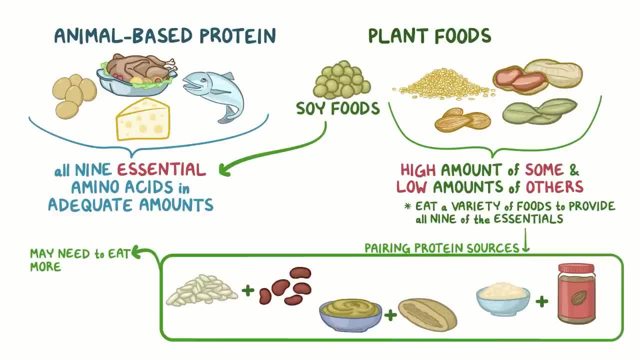 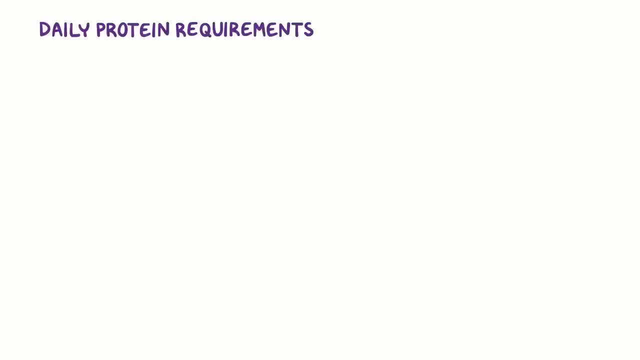 amount of protein and amino acid profile provided by animal-based proteins. Generally speaking, daily protein requirements are based on studies that estimate the minimum amount of protein needed to avoid a progressive nitrogen loss, The World Health Organization guidelines and the US Recommended Dietary Allowance each. 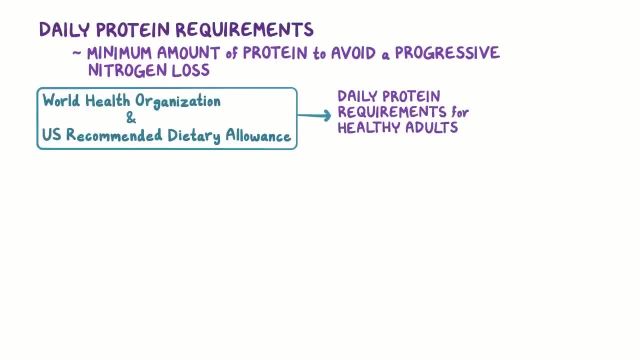 estimate that daily protein requirements for healthy adults are about 0.8 grams per kilogram of body weight. Protein recommendations per day vary by age as well. Children 1-3 years of age are recommended to get 13 grams. For ages 4-8, 19 grams are recommended. 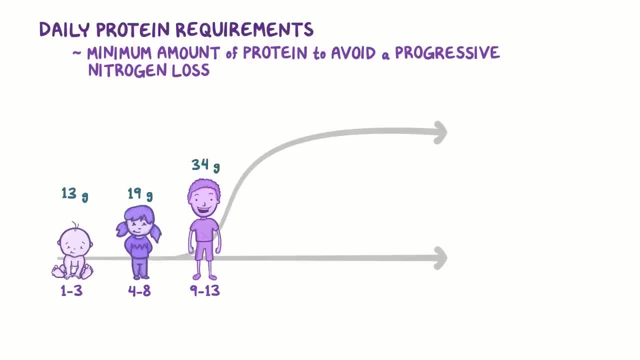 And between ages 9-13,, 34 grams are recommended. Whether a person is male or female also impacts protein needs. Females ages 14 and above are recommended to get 46 grams of protein per day. Males age 14-18, need slightly more- about 52 grams per day. 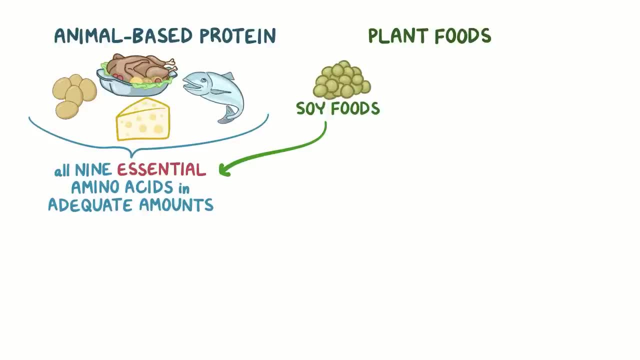 acids in adequate amounts. Most other plant foods, including whole grains, legumes, nuts and seeds, have high amounts of some amino acids and low amounts of others. Hearing this, it might be easy to assume that animal-based foods provide more protein than 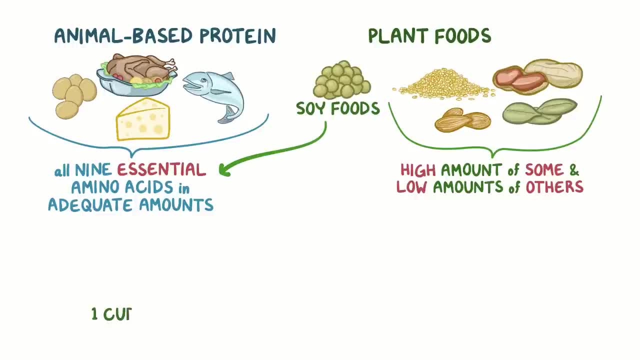 plant-based ones. But, as it turns out, a cup of tofu has the same number of grams of protein as three ounces of steak, chicken or fish, And half a cup of lentils has more grams of protein than an egg. And not all plant foods are low in the same amino acids, so eating a variety of plant-based 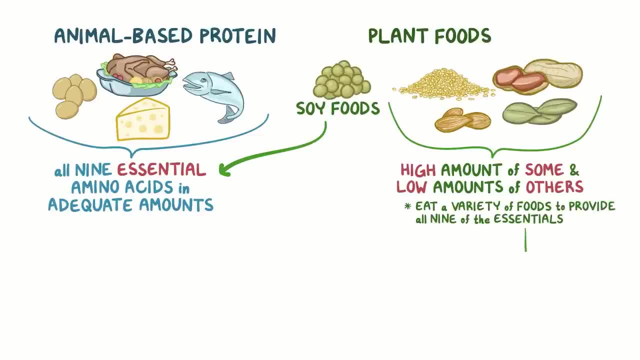 foods can provide all nine of the essentials, For example, pairing protein sources like rice and beans or hummus and pita bread or oatmeal topped with almond butter. However, in terms of volume, it may be necessary to eat more plant-based foods to get a similar. 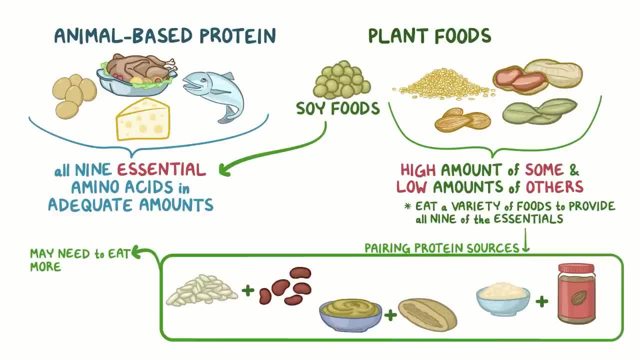 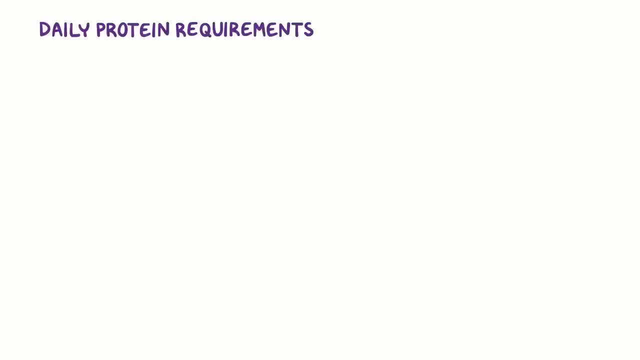 amount of protein and amino acid profile provided by animal-based proteins. Generally speaking, daily protein requirements are based on studies that estimate the minimum amount of protein needed to avoid a progressive nitrogen loss, The World Health Organization guidelines and the US Recommended Dietary Allowance each. 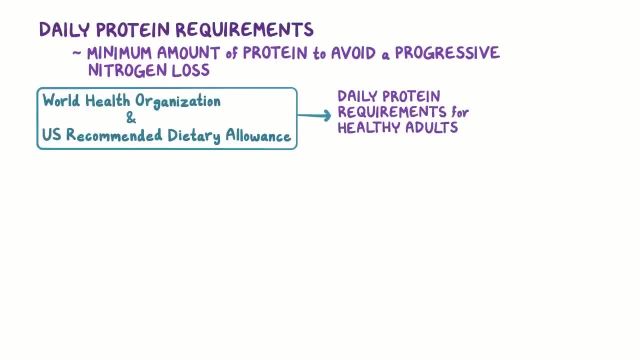 estimate that daily protein requirements for healthy adults are about 0.8 grams per kilogram of body weight. Protein recommendations per day vary by age as well. Children 1-3 years of age are recommended to get 13 grams. For ages 4-8, 19 grams are recommended. 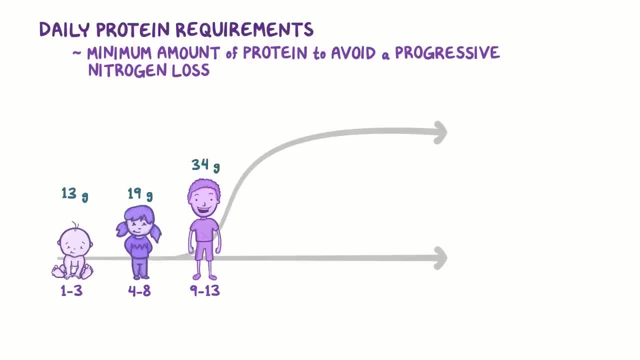 And between ages 9-13,, 34 grams are recommended. Whether a person is male or female also impacts protein needs. Females ages 14 and above are recommended to get 46 grams of protein per day. Males age 14-18, need slightly more- about 52 grams per day. 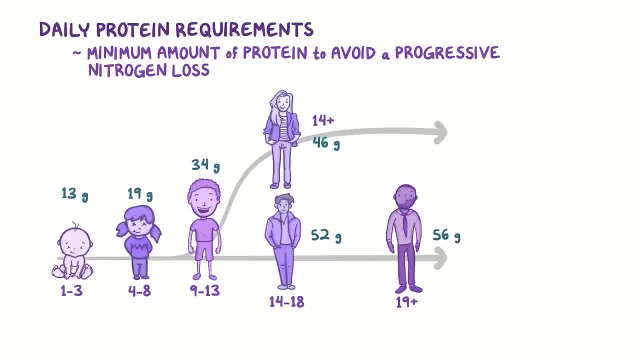 And males 19 and older are recommended to get 56 grams per day. Some groups, like pregnant and breastfeeding women, as well as athletes, have elevated needs, And older adults may also benefit from eating more protein. Getting the right amount of protein per day can be achieved in multiple ways. 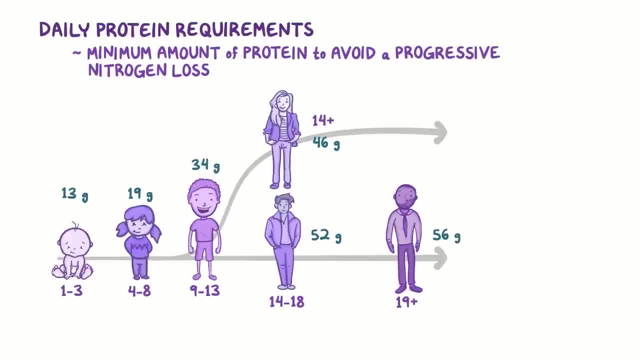 And males 19 and older are recommended to get 56 grams per day. Some groups, like pregnant and breastfeeding women, as well as athletes, have elevated needs, And older adults may also benefit from eating more protein. Getting the right amount of protein per day can be achieved in multiple ways. 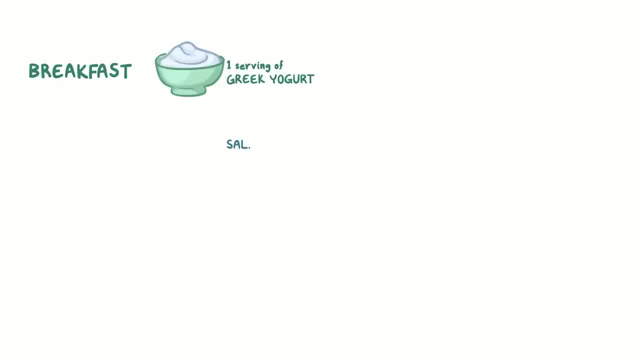 For example, one serving of Greek yogurt with breakfast, a salad topped with 3 ounces of chicken for lunch and 3-4 ounces of fish at dinner provides about 64 grams of protein. Getting the same amount of protein could also be achieved by eating a cup of tofu scramble. 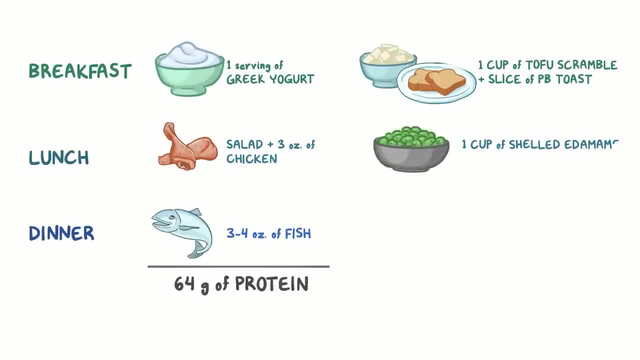 and a slice of peanut butter toast for breakfast, a cup of shelled edamame with lunch and one cup of lentils and brown rice at dinner, which also offers about 64 grams of protein in total. Now, the fact is that it's still unclear what an optimal amount of protein is, and the research 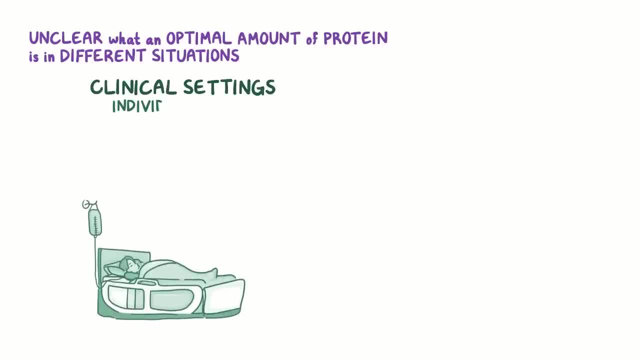 is ongoing In clinical settings. there are certain individuals who may be at risk for a protein deficiency, including patients with malnutrition, trauma and burn injuries, as well as various conditions impacting nutrient absorption. So what are the most common causes of protein deficiency? 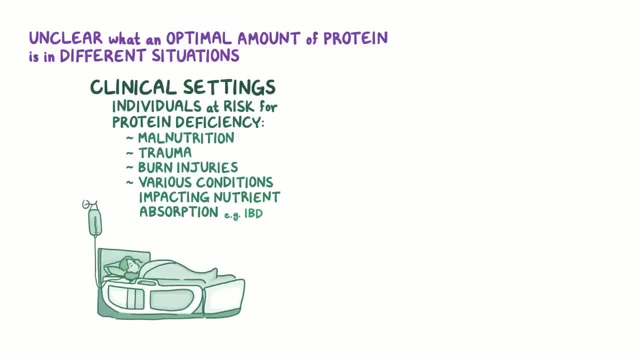 The most common cause of protein deficiency is a lack of protein. These individuals may have increased protein needs compared to the general population. Except for certain circumstances like kidney disease, there usually isn't a health risk associated with eating a lot of protein, because our bodies are able to process it. 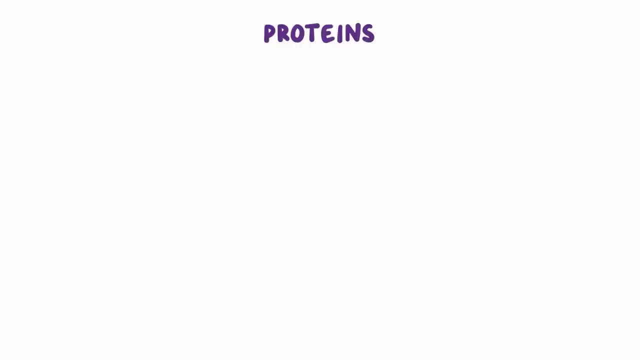 Alright, as a quick recap, protein is a cornerstone of the human diet and a major component of our bodies. There are 5 non-essential, 6 conditionally essential and 9 non-essential. We need to get essential amino acids from our diet. 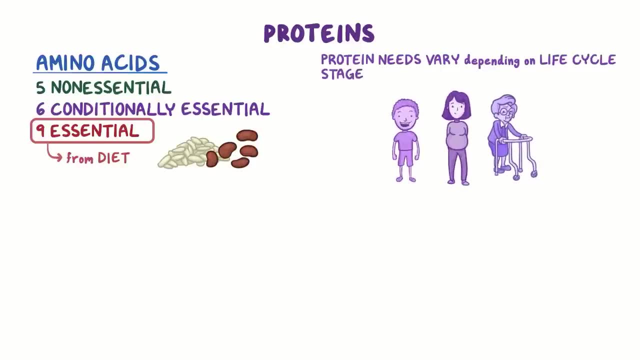 Protein needs vary depending on life cycle stage, level of physical activity and health status. Some health conditions may put people at risk for protein deficiency or increased protein needs. Everyone, whether omnivorous, vegetarian or vegan, can get enough protein by eating. 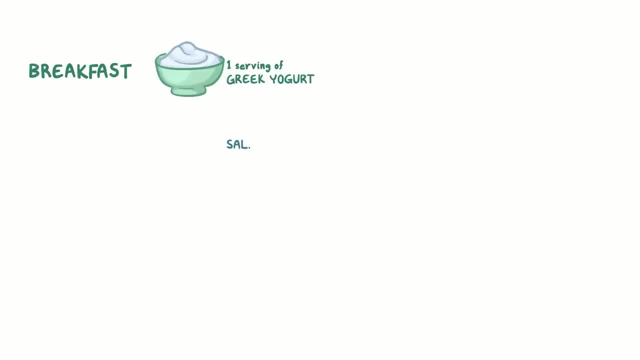 For example, one serving of Greek yogurt with breakfast, a salad topped with 3 ounces of chicken for lunch and 3-4 ounces of fish at dinner provides about 64 grams of protein. Getting the same amount of protein could also be achieved by eating a cup of tofu scramble. 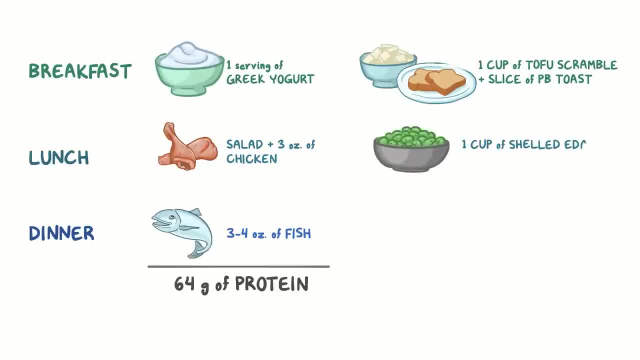 and a slice of peanut butter toast for breakfast, a cup of shelled edamame with lunch and one cup of lentils and brown rice at dinner, which also offers about 64 grams of protein in total. Now, the fact is that it's still unclear what an optimal amount of protein is, and the research 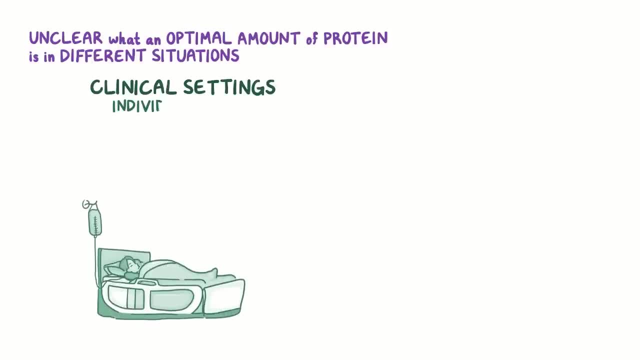 is ongoing In clinical settings. there are certain individuals who may be at risk for a protein deficiency, including patients with malnutrition, trauma and burn injuries, as well as various conditions impacting nutrition. These individuals may have increased protein needs compared to the general population. 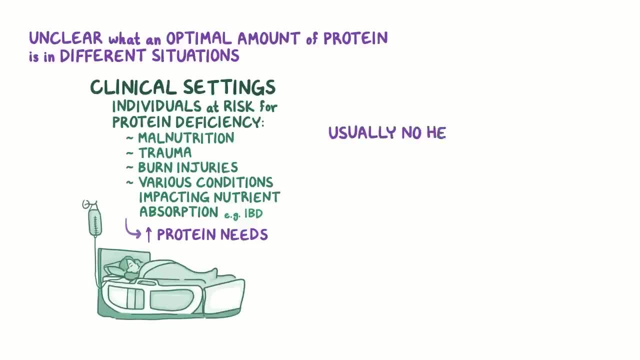 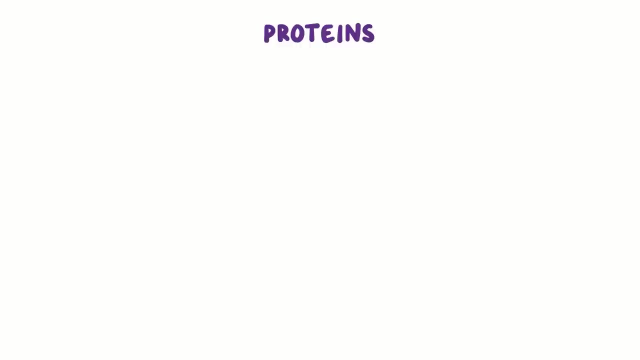 Except for certain circumstances like kidney disease, there usually isn't a health risk associated with eating a lot of protein, because our bodies are able to process it Alright. as a quick recap, Protein is a cornerstone of the human diet and a major component of our bodies. 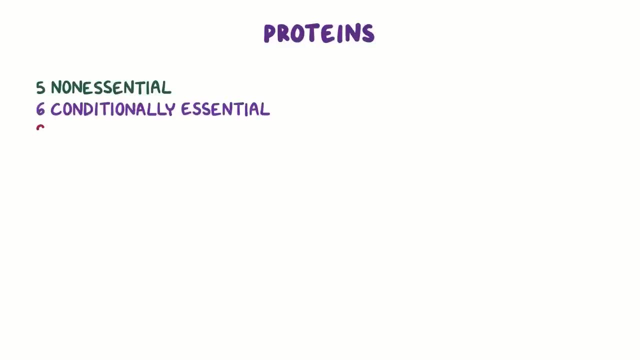 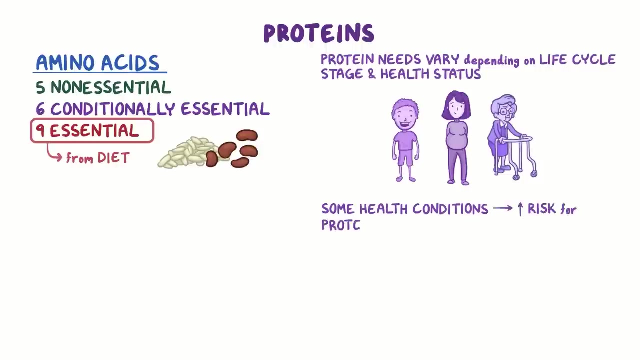 There are 5 non-essential, 6 conditionally essential and 7 non-essential. We need to get essential amino acids from our diet. Protein needs vary depending on life cycle stage, physical activity and health status. Some health conditions may put people at risk for protein deficiency or increased protein. 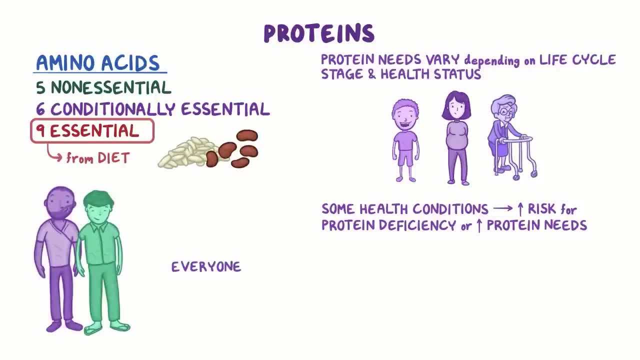 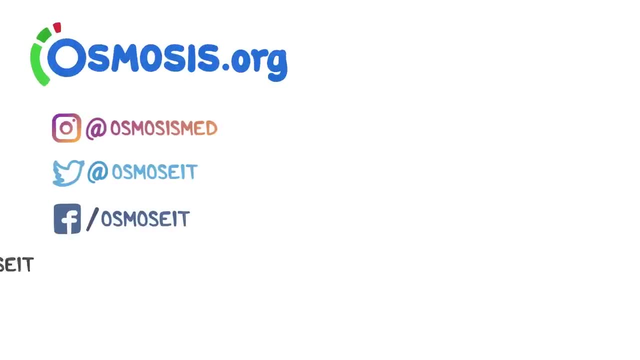 needs. Everyone, whether omnivorous, vegetarian or vegan, can get enough protein by eating a variety of foods. Some people may get a protein deficiency by eating a lot of protein and others may get that because they are busy eating a lot of protein like they need. Get more protein. Eat more. Don't get enough. Don't get too full. Eat less. Take more. Don't get too full. Don't get too full. Don't get too full in a day. Eat less. Don't get too full. Don't get too full on a day. Eat less. Jamie, I will ask you this real quick: What are the causes of protein deficiency and what can the sana function do to contribute to protein deficiency? There are three types of protein deficiency. Here is some examples: Lactamine: